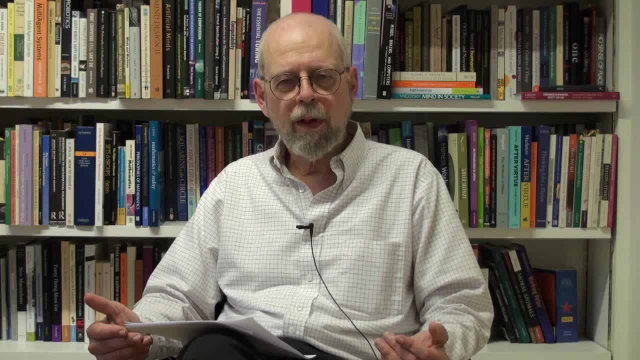 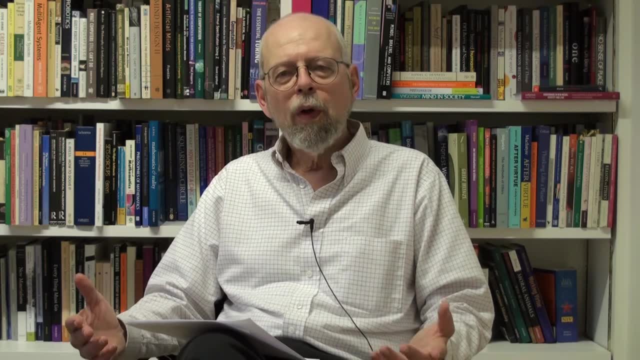 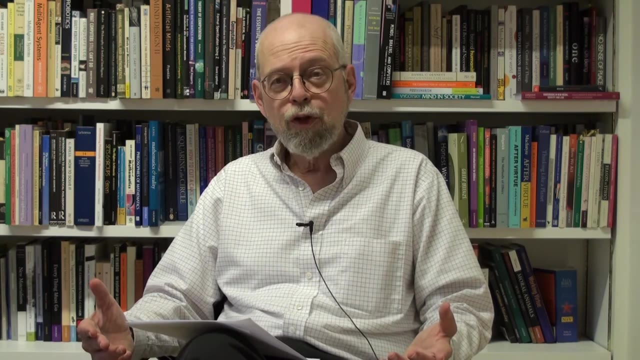 interact with the dependent variable in much more complex ways. So the problem for a multiple regression analyst is to figure out what exactly is happening, And that deals with the question of diagnostics. Diagnostics are heavily visual. We're going to spend a lot of time looking. at visual sort of pictures of relationships between the two And we're going to spend a lot of time looking at visual sort of pictures of relationships between the two And we're going to spend a lot of time looking at visual sort of pictures of relationships between. 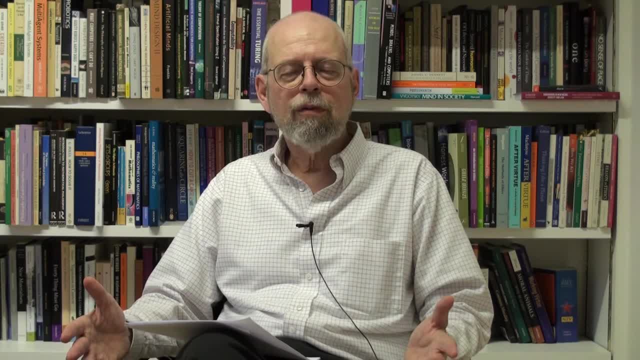 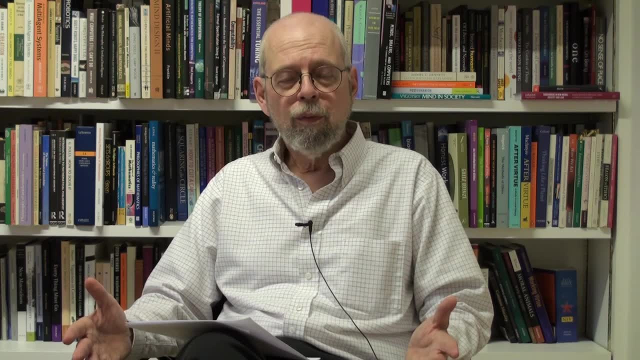 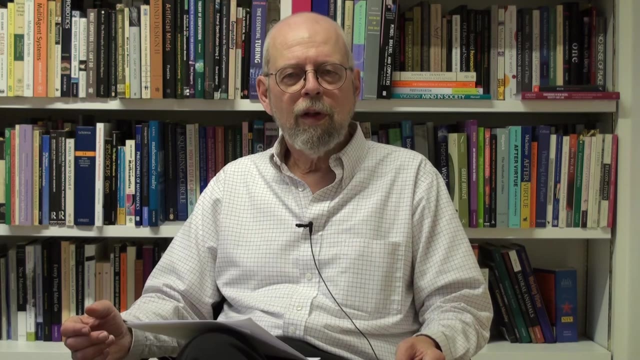 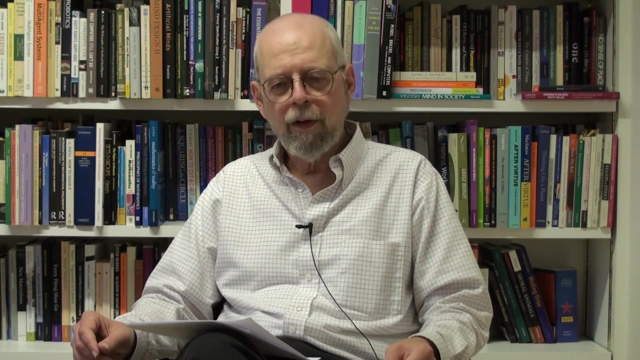 variables. We'll look at visual pictures of distributions, We'll look at how to diagnose normality or lack of normality in the distribution of the variables And we'll also look at some numerical diagnostics for things like the relationships between independent variables. which is the technical name for this is collinearity. The bottom line on all of this is that the 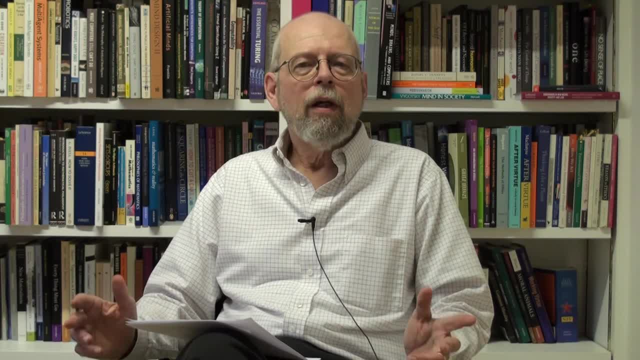 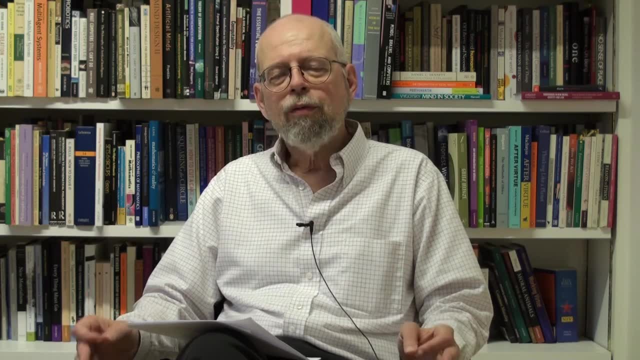 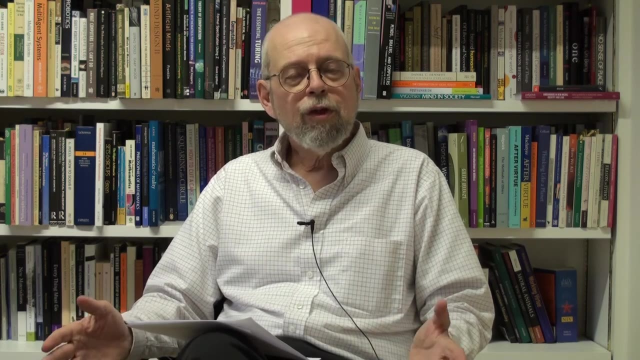 course is a fundamental one for social scientists. It deals with a fundamental technique. It prepares you for all sorts of other statistical models. Multiple regression is well understood and the sort of issues there are well understood. When you move beyond multiple regression they're not nearly so well understood. But the problems, the same problems, occur If you know how to. 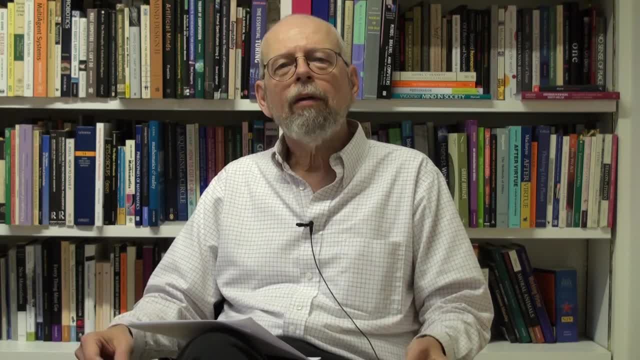 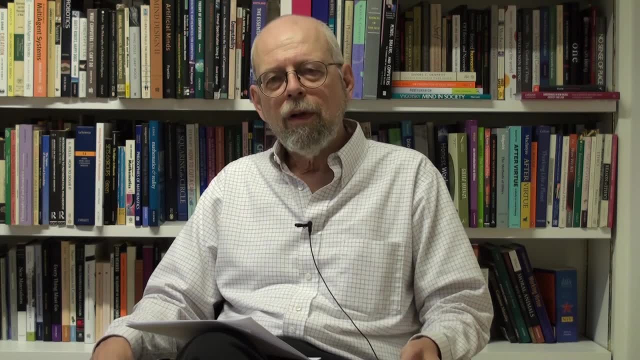 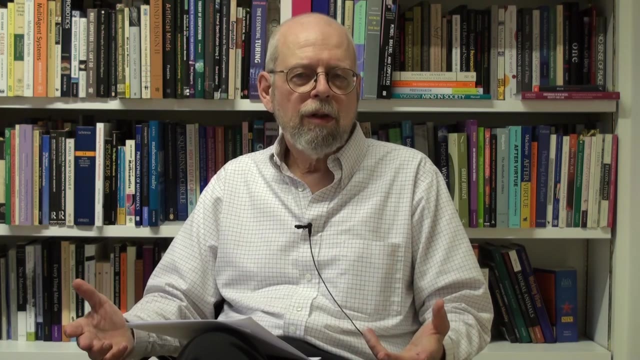 handle those problems in a multiple regression environment you're going to be able to solve them environment. it's very straightforward to transfer that knowledge to other environments with other kinds of statistical models. So this course forms a real basis for almost anything else you'll do with multivariate models in. 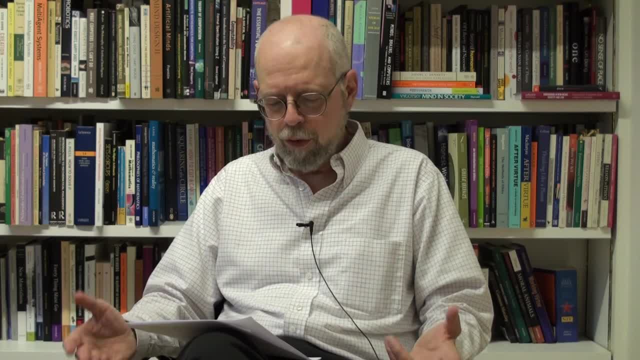 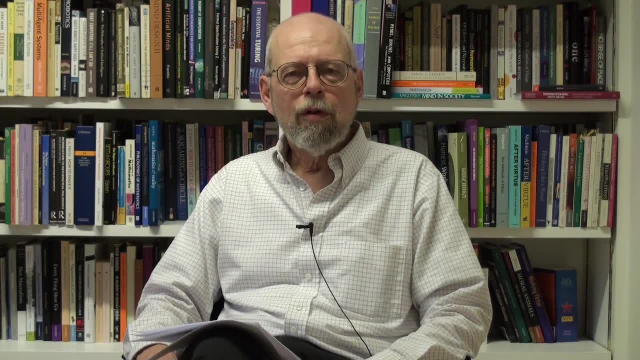 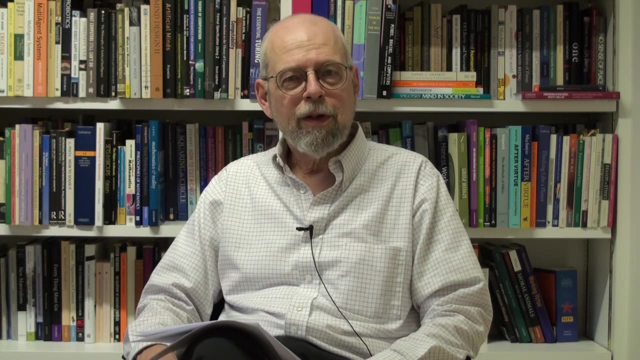 the social sciences. It's a fundamental part of the social sciences. in that sense, If you're doing a quantitative thesis, this course will give you the sort of tools you need to produce high quality analysis and high quality results. I hope to see you next term.